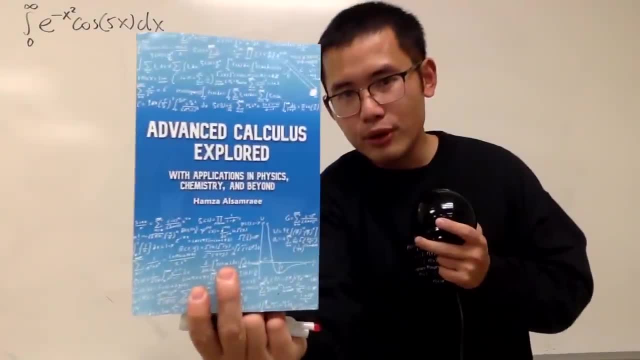 First of all, let me tell you I got this question from this book right by DailyMath, as I told you guys last time. So check that out if you would like. I will have the link in the description for your convenience. 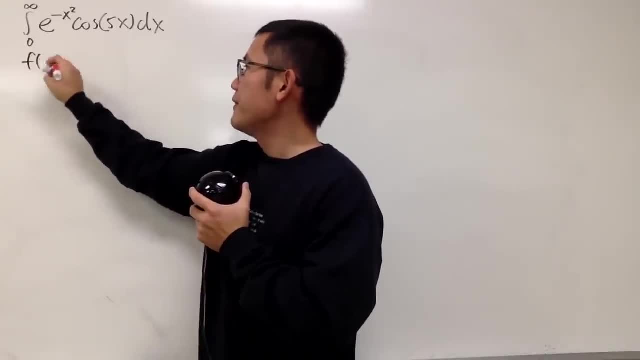 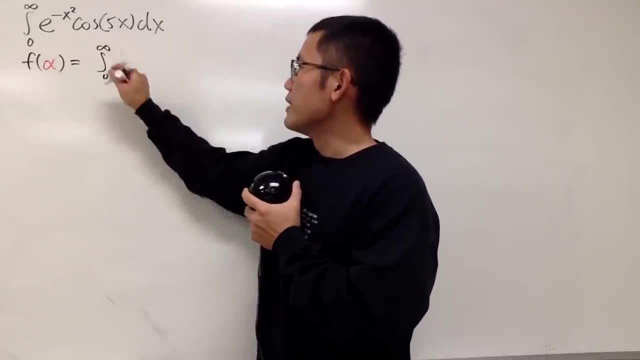 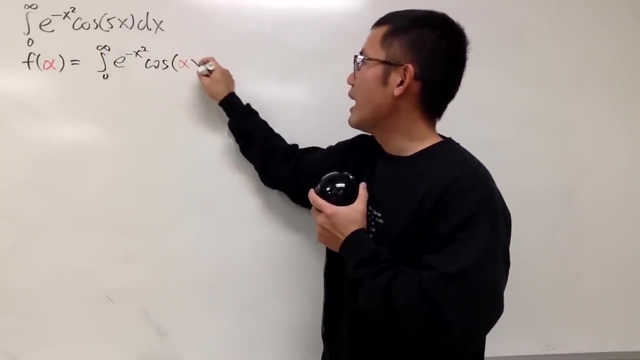 Alright, I'm going to start off by calling this to be f and let's call the parameter alpha And this right here. we'll just write it as integral from 0 to infinity, e to the negative, x squared cosine, but instead of the 5, we are going to put down alpha and then x, dx. 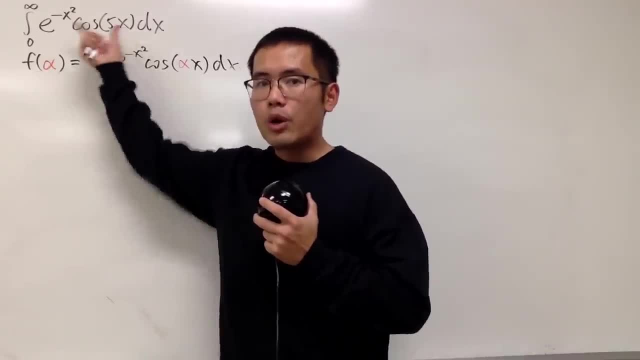 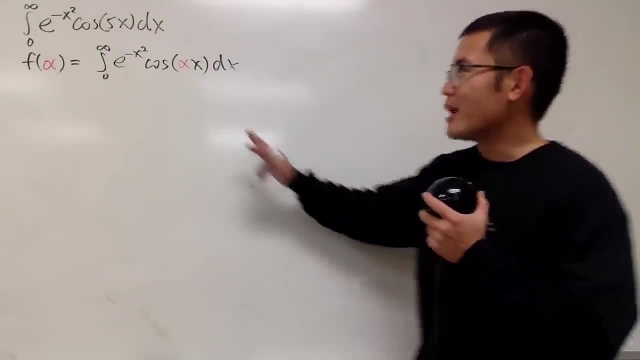 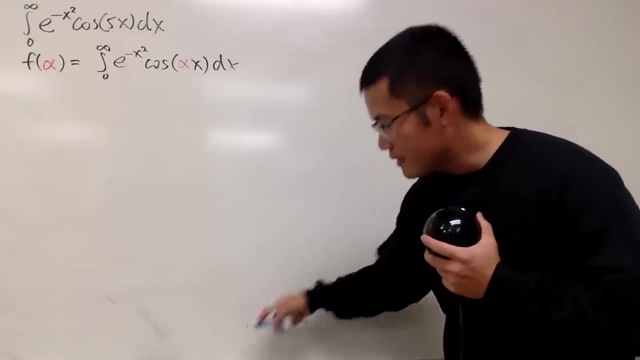 Because look at, this f of 5 is exactly our original integral And in fact, after we finish the procedure right here, you will see you can compute this kind of integral with whatever number you want, right here. Very nice, Okay, now here is the time to do our derivative. 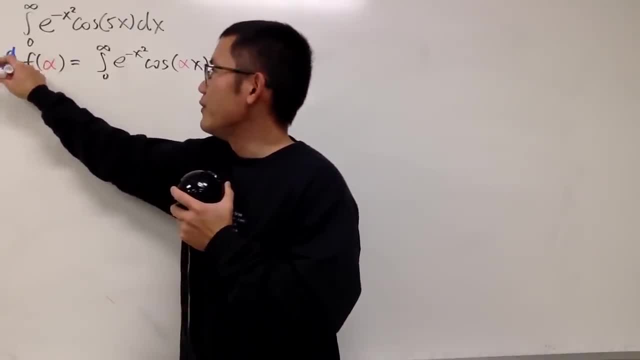 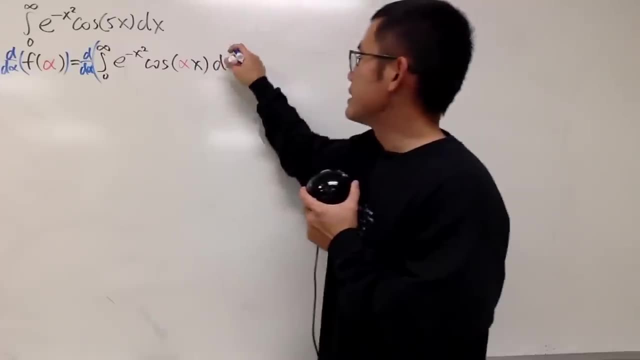 On the left-hand side and also the right-hand side. we are going to differentiate both sides With respect to alpha. So let's put down dd alpha on both sides. On the left-hand side, I'm just going to write down the derivative in the prime notation. 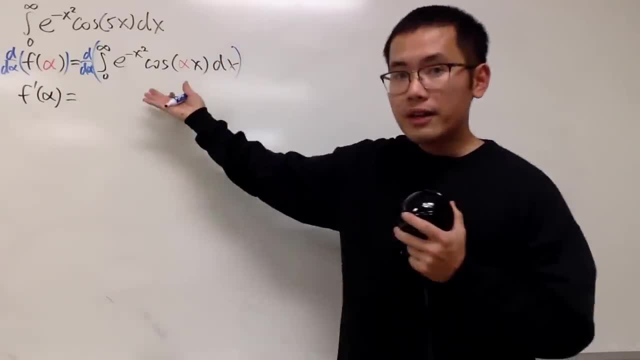 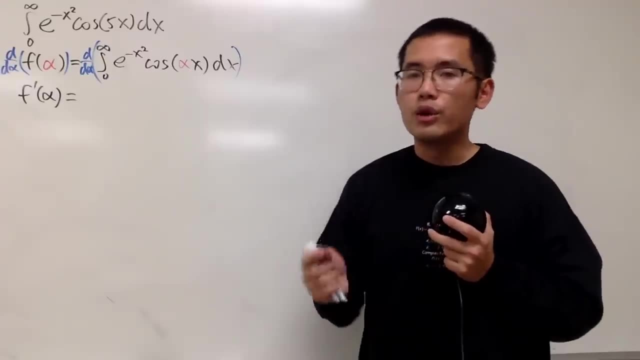 So here is f prime of alpha. However, on the right-hand side, we will have to bring the derivative inside of the integral And let's call the famous technique, or you can also call that to be the differentiation under the integral sign. 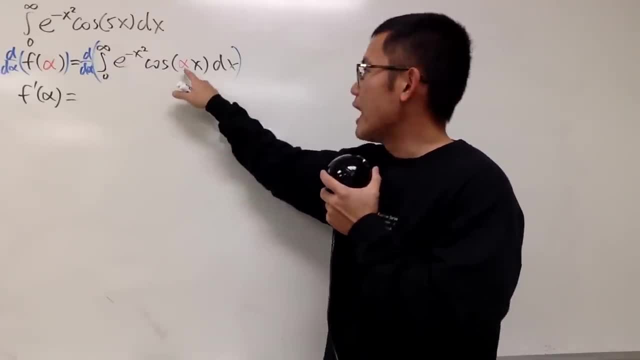 When you bring this in, because inside here we have the derivative, we have the integral And here we have both the alpha and also the x. We have two things right. So be sure you change that to partial derivative. 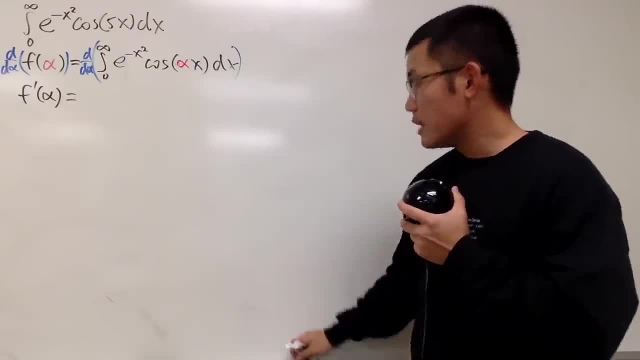 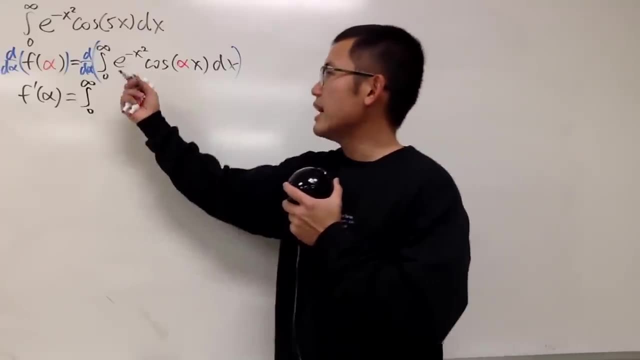 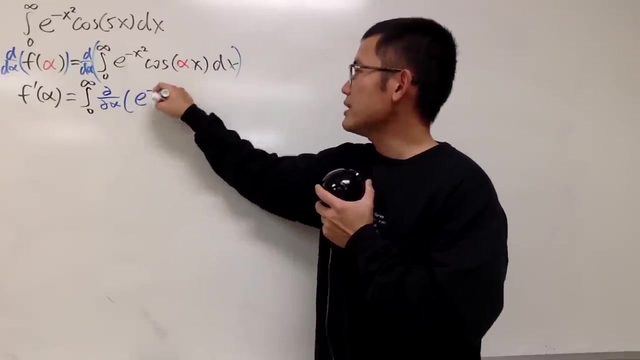 And let me just make the alpha slightly more clear for you guys. Alright, so here is the integral from 0 to infinity, And then again we are looking at this as partial with respect to alpha, and then all that. So we have e to the negative x squared cosine of alpha x. 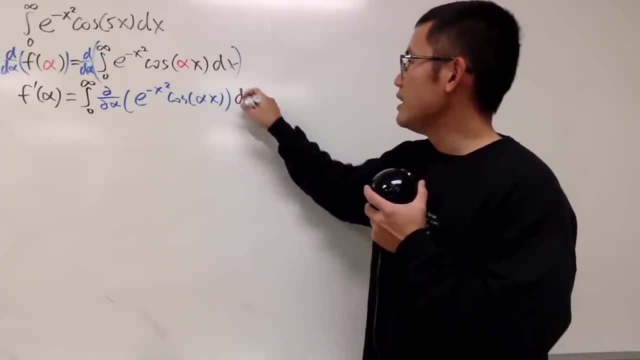 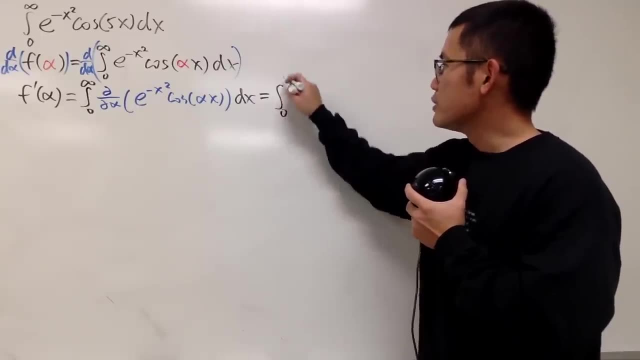 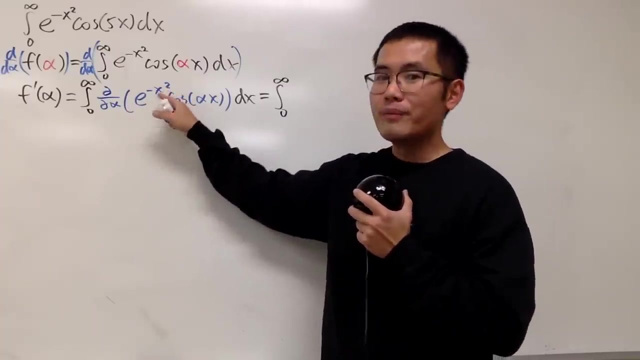 And then, of course, on the outside We still have the dx like this: Now we are going to work this inside out, So have a look right here. Integral from 0 to infinity. In the alpha world, x is a constant, so is e to the negative, x squared. 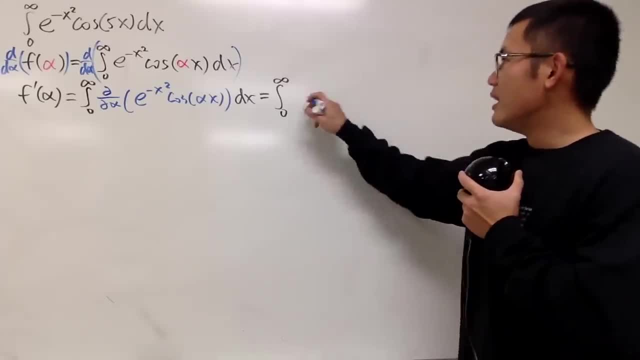 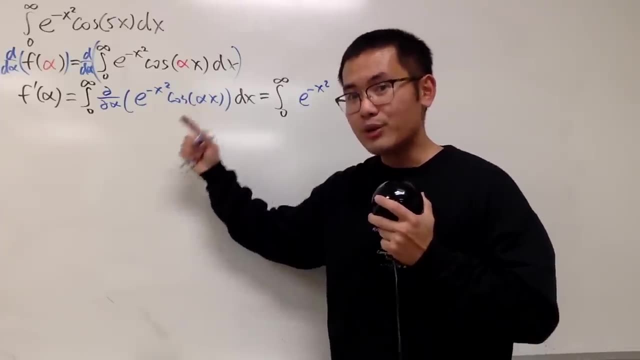 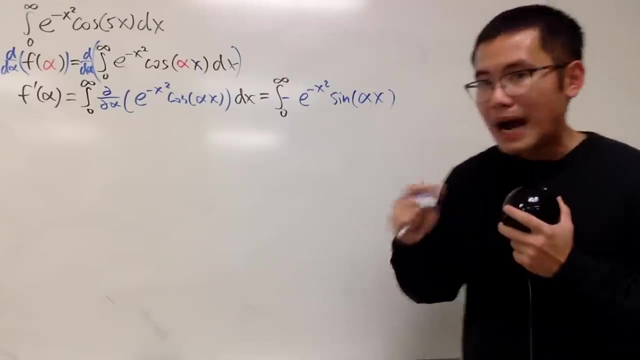 Of course we will just write that down first. Here is the e to the negative x squared Now, as we can see, alpha is inside of cosine. So we are going to differentiate cosine And that will give us negative And the input stays the same. but Chen Lu says we have to multiply by the derivative of the inside. 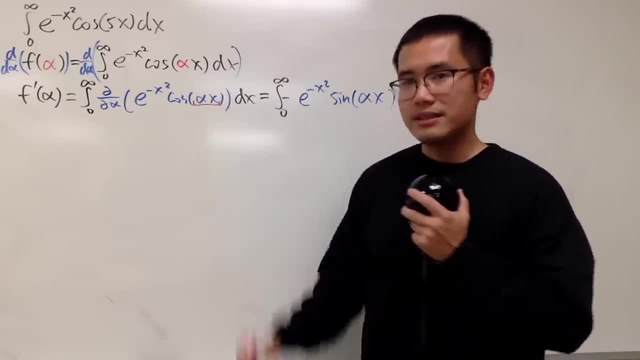 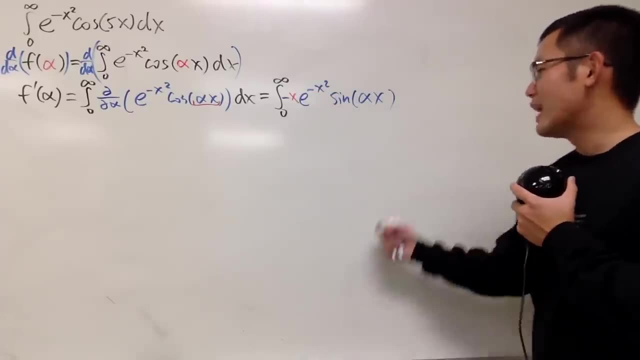 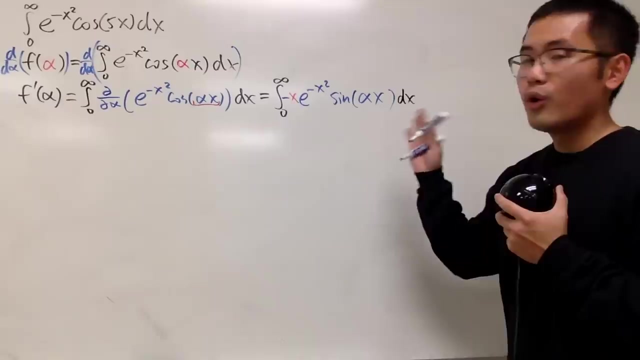 With respect to alpha: alpha is the variable, x is the constant, so we have to multiply by x. right here, Very nice. And of course, this right here. we still have the dx on the very outside, like this. Alright, now, this is so wonderful. 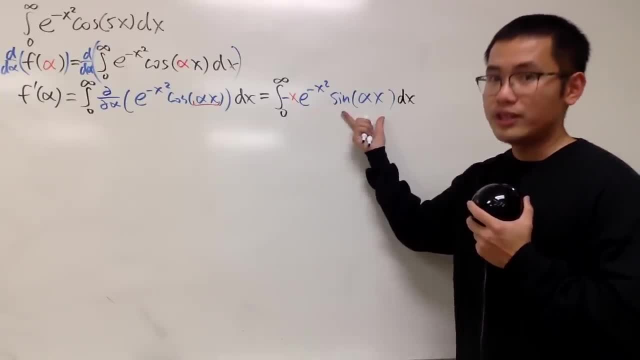 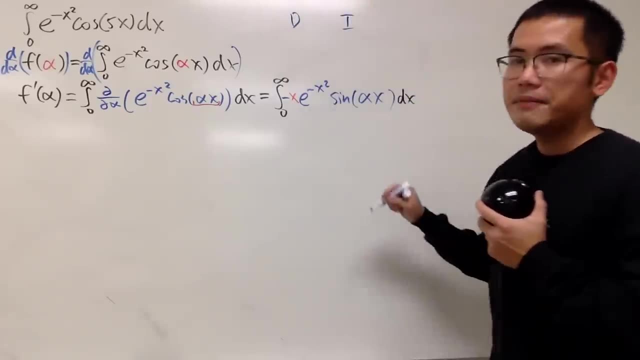 Because we can integrate this part And we can, of course, differentiate this part. So let's go ahead and do the di-theta for the integration by parts. I will put it down right here: b and also the i Plus minus to get ready. 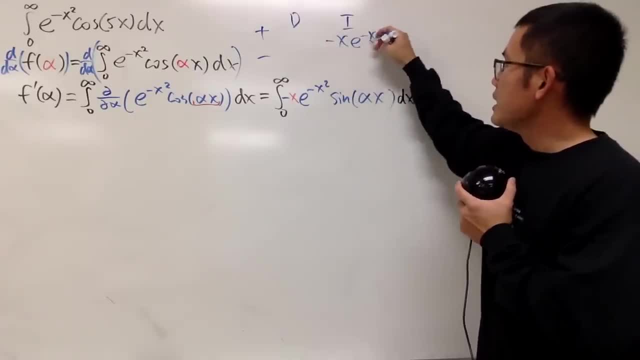 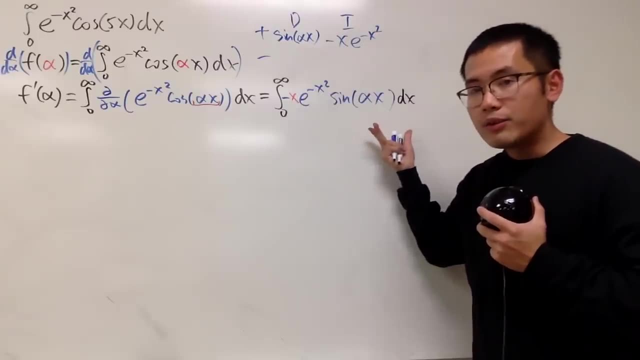 Integrating this part: negative x e to the negative x squared. differentiating sine of alpha x. Keep in mind, though, we have to do the work with respect to x. Right, we are in the x world now. So differentiating sine of alpha x. 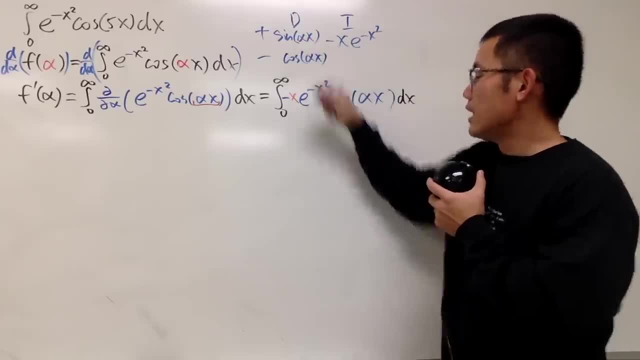 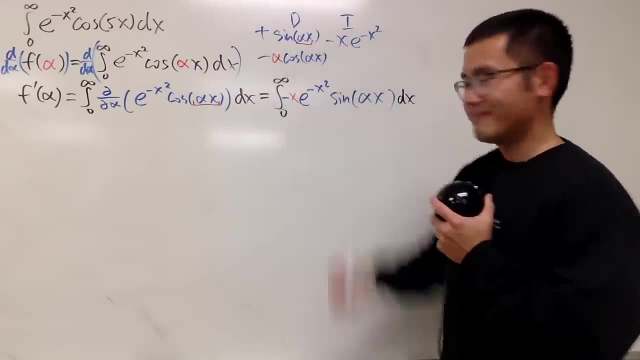 We get cosine of alpha x, and then the Chen Lu says: multiply by the derivative of alpha x with respect to x, This time we multiply by alpha. And then for this one we are just going to do the integral in your head. 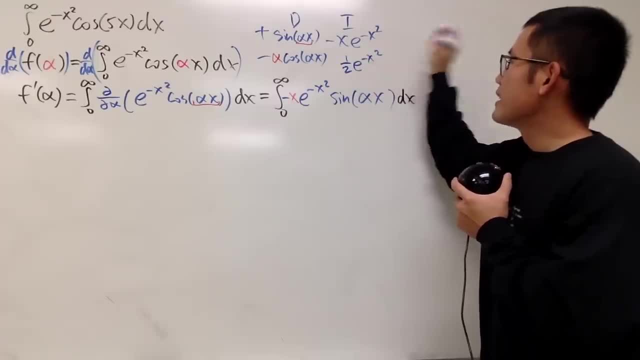 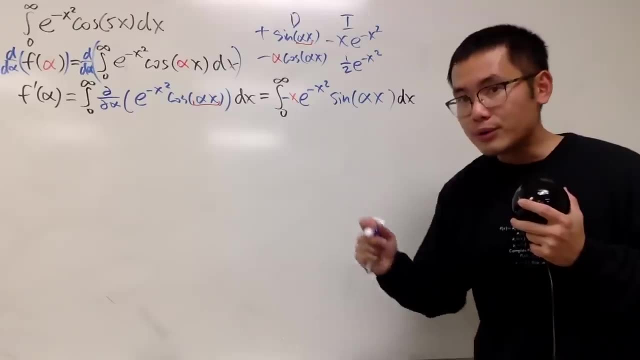 We end up with 1 half e to the negative x squared. thanks to this x right here on the outside, We can just do u-theta for that. Very nice, Now to continue. of course we know this times that it's the first part of the answer. 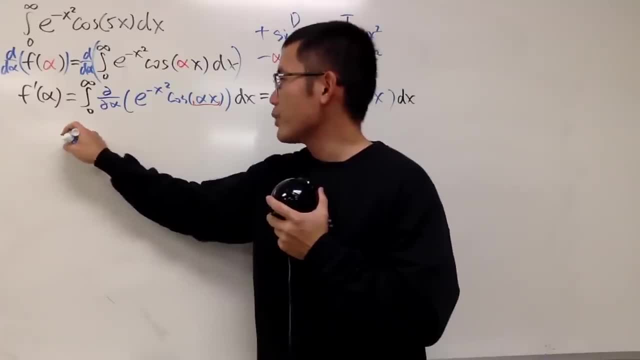 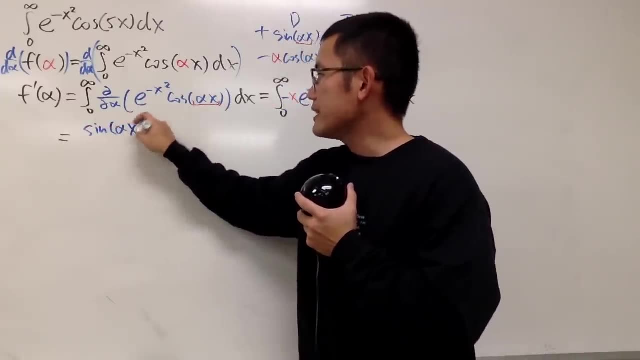 So I'm going to just come back right here and we are going to write it down. Well, I'm going to put this on the top. So we have sine of alpha x and then over we have the 2, and also bring that down because of the negative exponent. 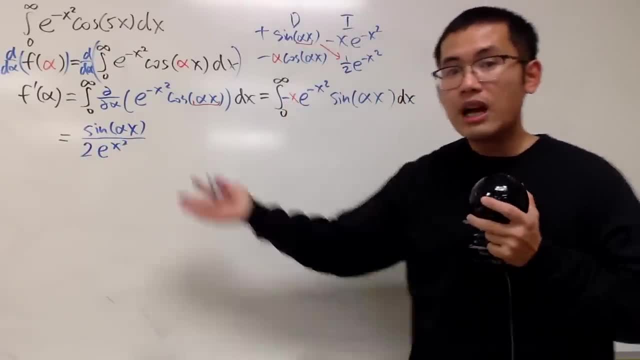 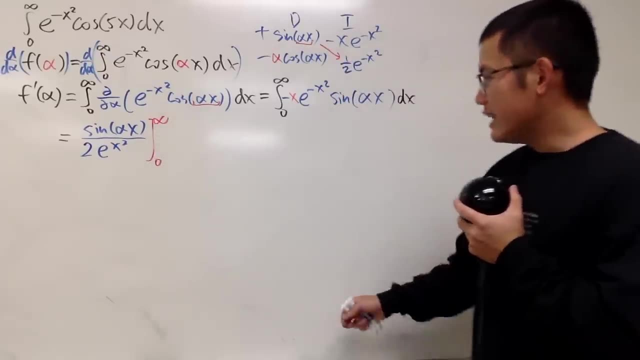 So we have 2e to the positive x squared. That's the first part of the answer. so don't forget to plug in, plug in right from 0 to infinity And then to continue. remember we have to multiply. 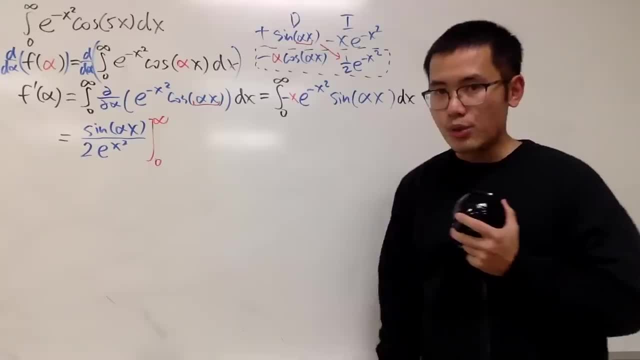 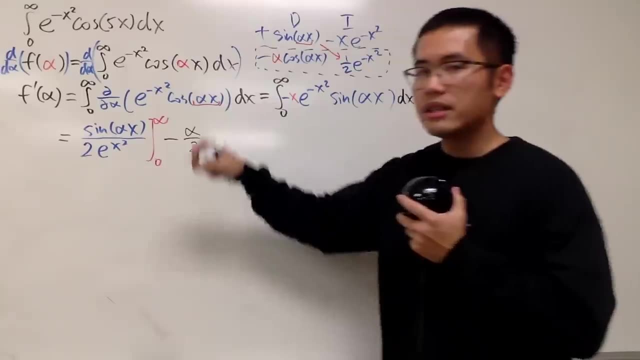 So we multiply this row and this right here is still an integral negative alpha, and then we have the 1 half. So let me just write down minus alpha over 2, the constant, in the front, and then put this and that inside of the integral right. 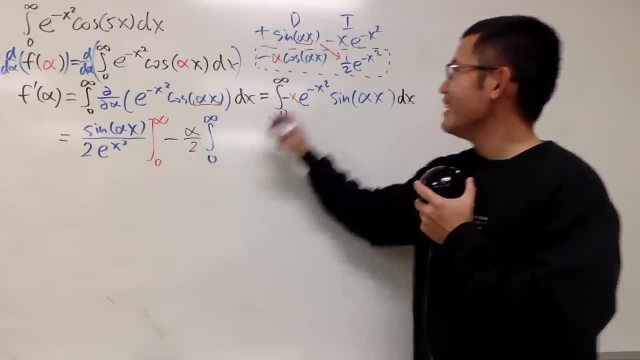 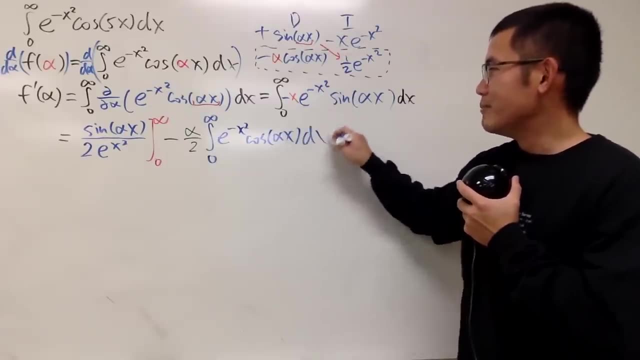 So we have the integral still going from 0 to infinity, and we have this first because, why not? And you'll see, we have a small deja vu, because doesn't this look familiar? Yes, it does, It's our f of alpha. 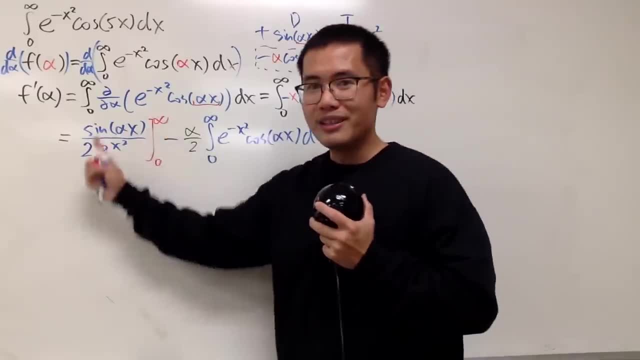 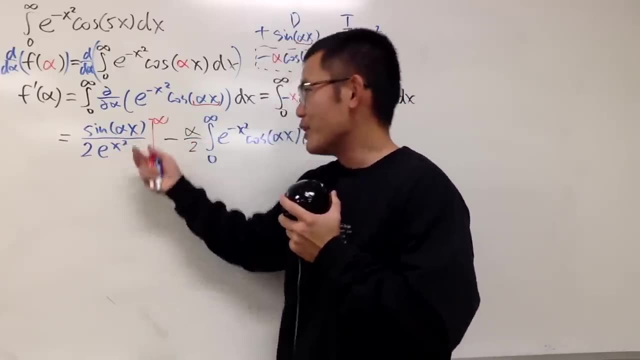 Alright, so now look at this. This right here is super nice, because the answer to this is 0.. When you put infinity to here, like e to the infinity, and then you square that man, the bottom is so much bigger than the top. 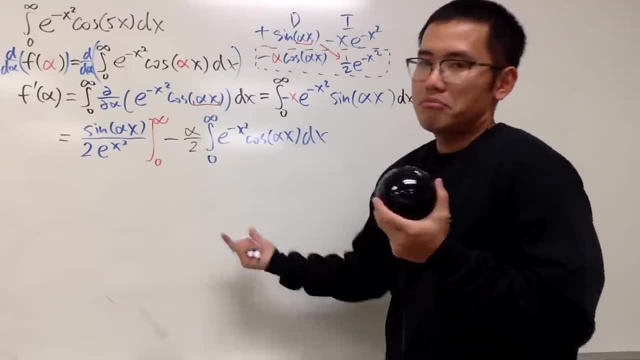 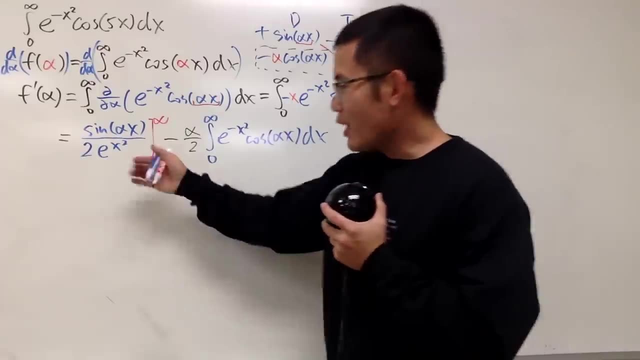 The top is at most 1, right Or negative 1, like, yeah Well, you get 0. And then when you put 0 into here, thanks to sine of 0, you get 0 as well. So we end up with. 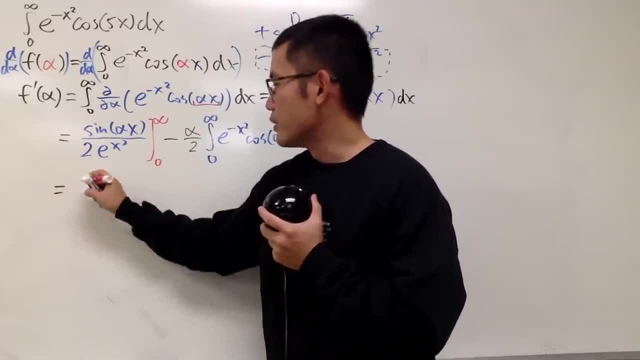 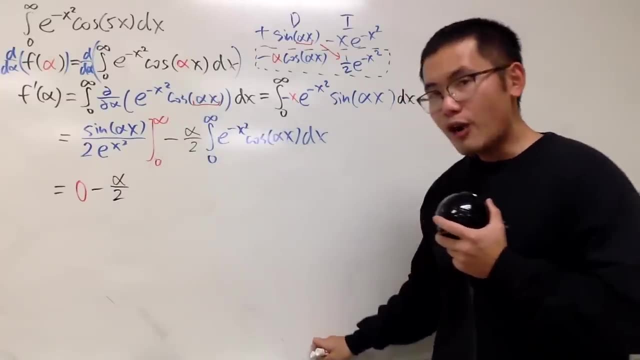 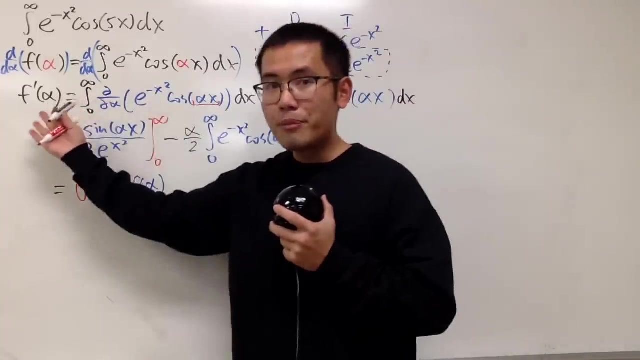 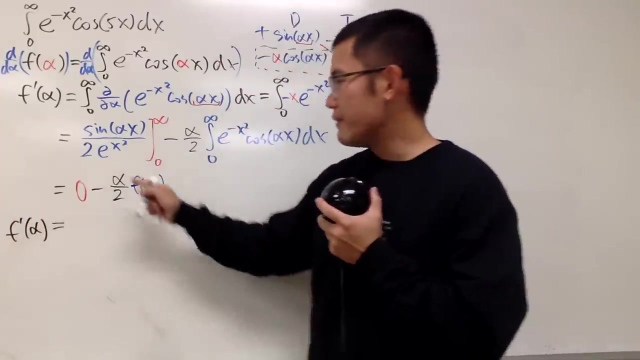 This, This right here we have 0, and then I will put down, minus alpha over 2, and this right here is our f of alpha. so we will of course just write that down. And now remember the left-hand side, we have f prime of alpha, and then on the right-hand side we have negative fish over 2 times f of alpha, like this right. 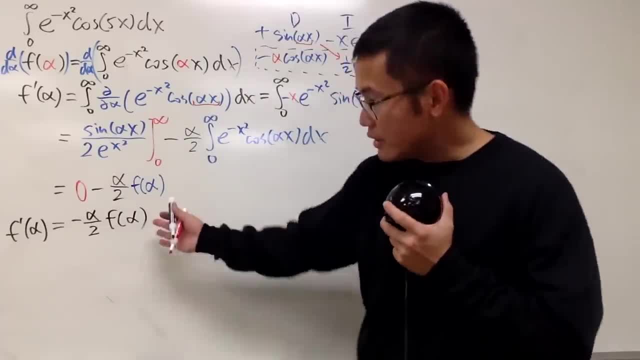 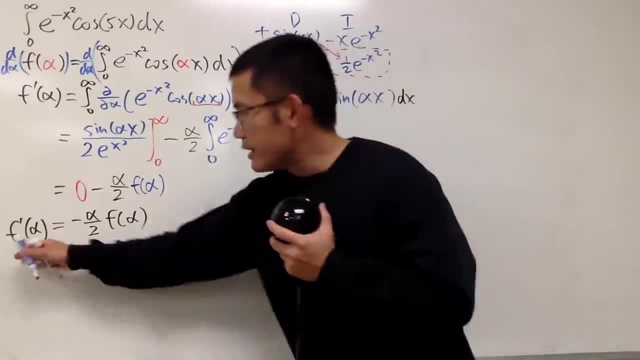 Yes, this right here is a differential equation, but, don't worry, This right here is a separable differential equation, so it's not so bad, And I'm going to just do the work right over there for you guys. I'm going to write this as df d alpha right. 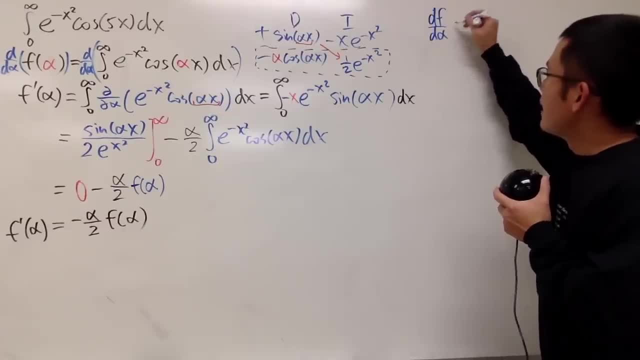 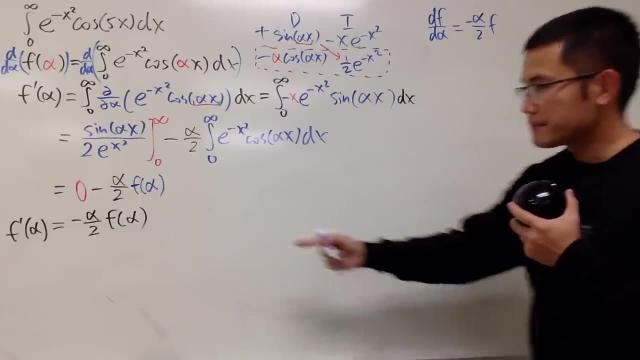 So df over d alpha And this right here is equal to negative alpha over 2, and then multiply by f, like this right, And then separate the variable. divide the f on both sides, multiply the d alpha on both sides. 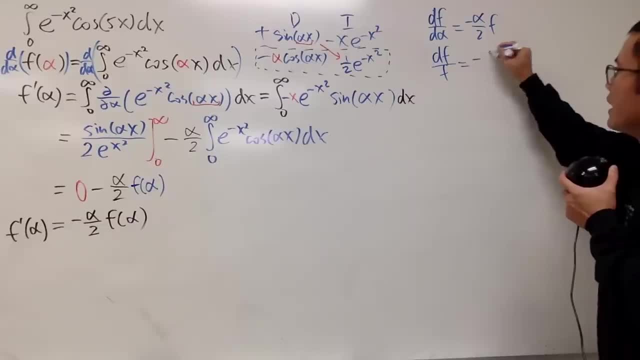 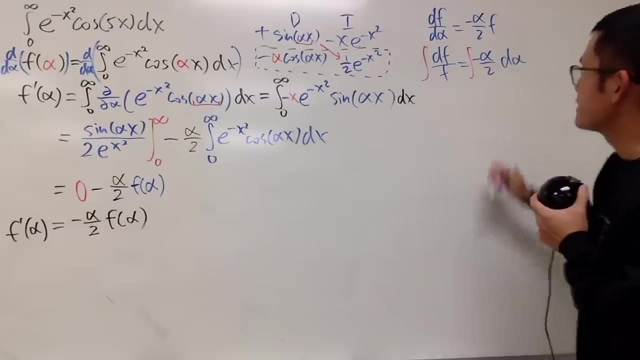 So we have, So we have, So we have df over f. this is equal to negative alpha over 2 times d alpha. And then, of course, we can integrate both sides. now, Very nice. The left-hand side: we get ln, absolute value of f plus a constant. but don't worry, just do it on the right-hand side. 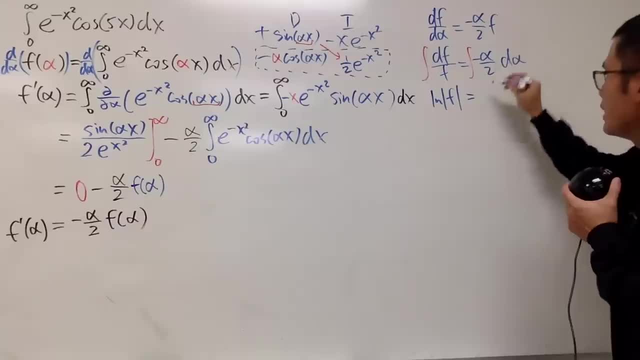 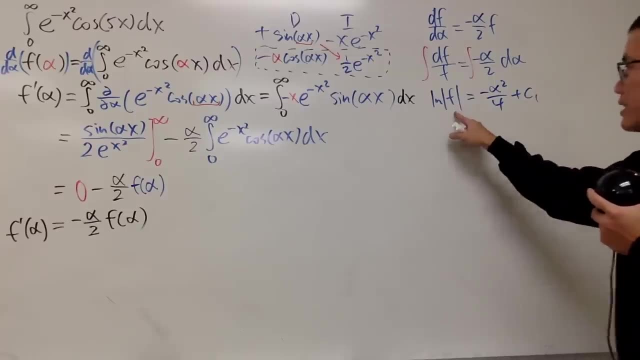 Integrating this. add 1 here, which you get 2, and then divide it by 2.. So we end up with negative alpha squared over 4, plus our first constant. Now to isolate f, let's do a lot of things in our head. 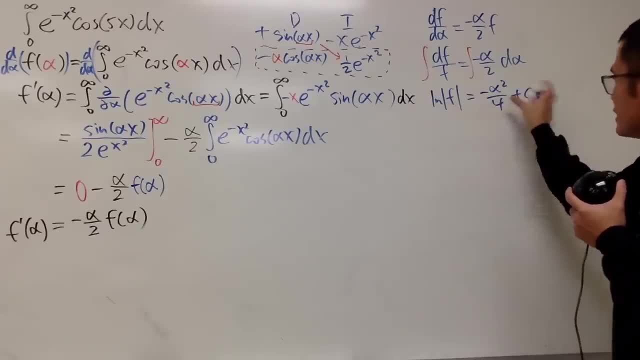 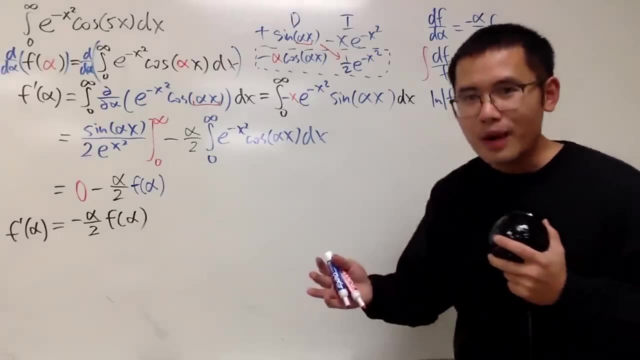 Do e to that power on both sides. e to this power is the same as saying e to this power times e to the c1. But c1 is a constant. e is a constant, c1, e just constant. e to the c1 is a constant, very nice. 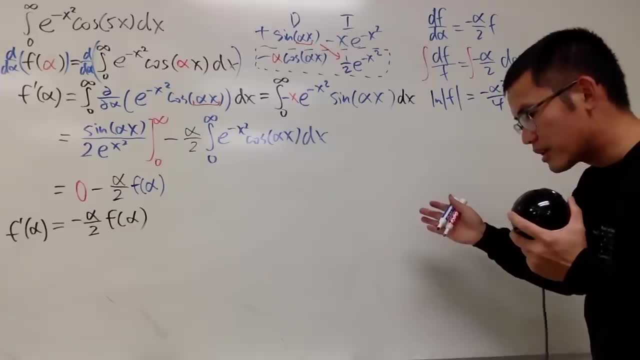 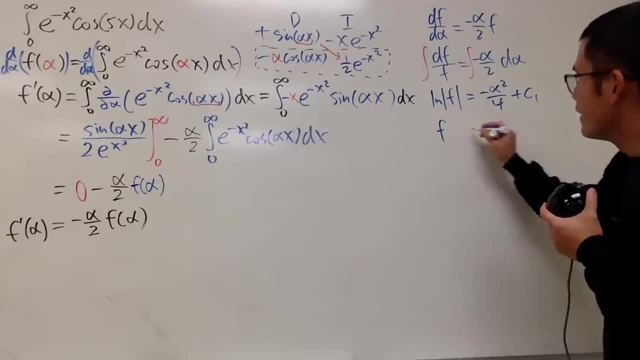 And then do the absolute value. You have to take it down of the absolute value. do the plus minus, so you have another constant. Anyway, I will just write this as f, That's equal to our constant. I'll just put it as c2.. 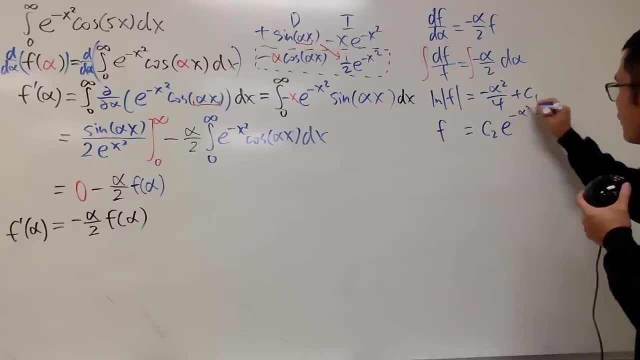 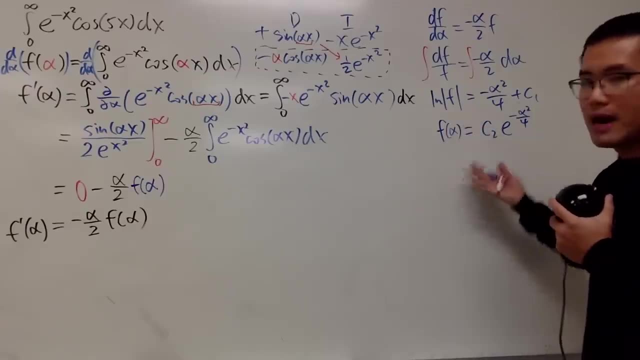 And then we have e to the negative alpha, squared over 4, like this right? Well, this is actually our f of alpha and we solve this differential equation. This is very nice, But the problem is that we have a c2 right here. 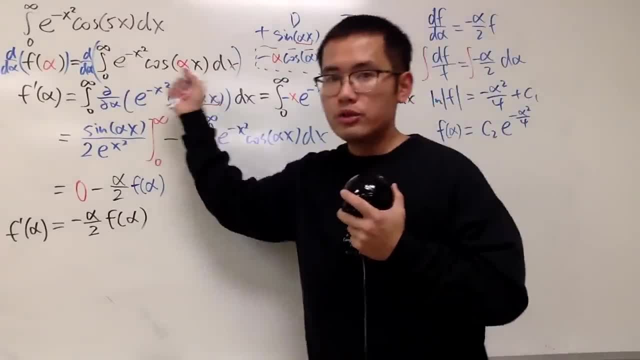 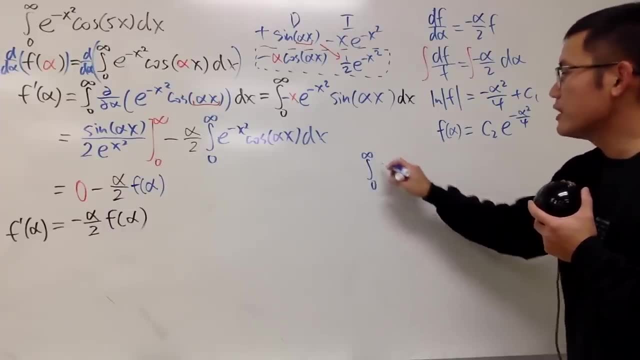 Oh well, this right here refers back to our original integral and hopefully we know something about that. So have a look. This right here is the same as a integral from c. So we have zero to infinity, e to the negative x squared cosine of alpha x, dx. 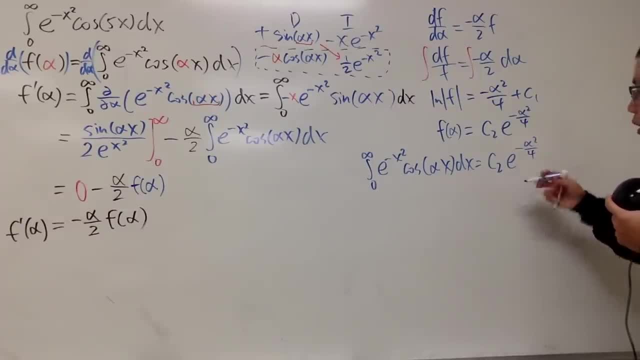 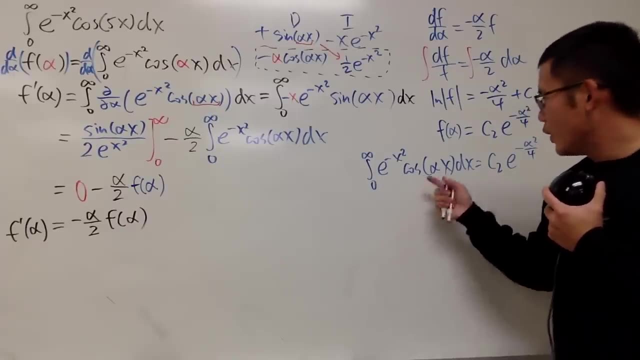 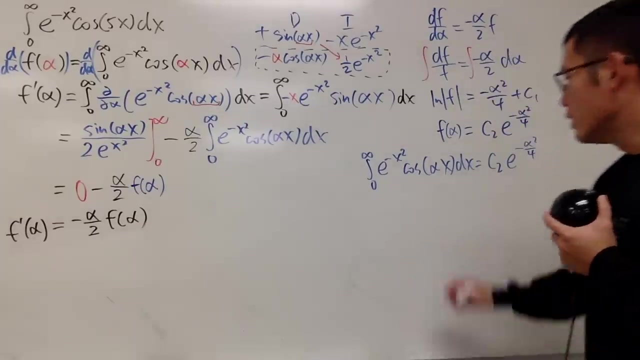 and this is equal to c2, e to the negative alpha squared over 4, like this. Well, what do we know about this? The truth is, we never liked the cosine of alpha x in the first place, right? So now let's think about how can we get rid of this. 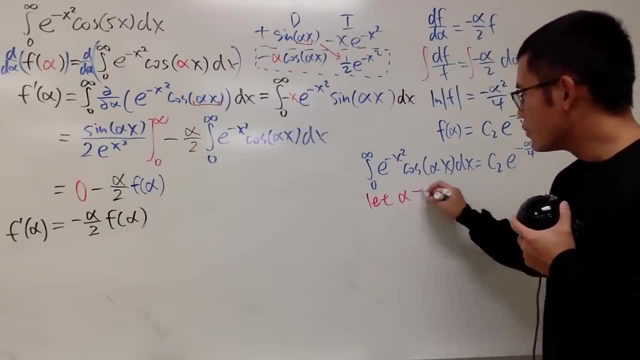 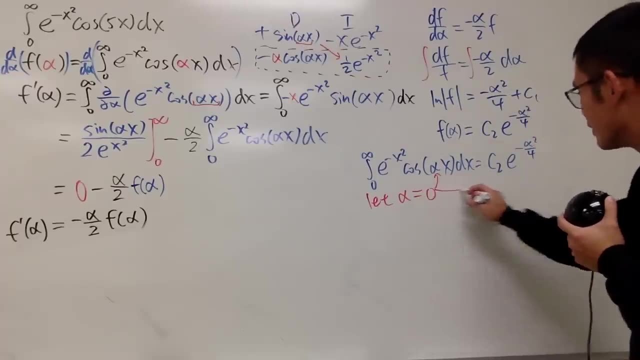 Oh well, in this situation, let's go ahead and let alpha to be zero, because if we put zero inside, cosine of zero is just going to be one. Very nice, And of course we can also put zero right here. 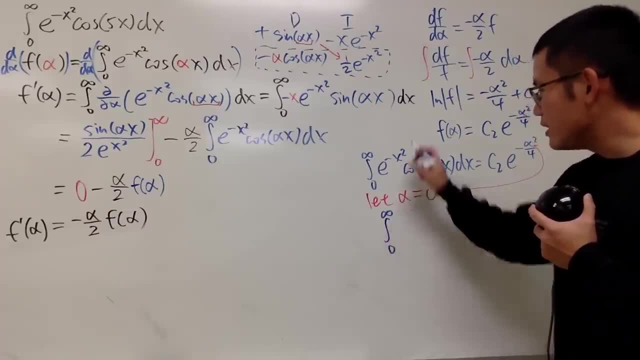 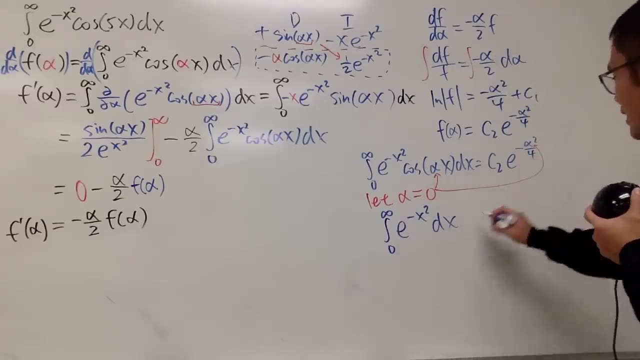 So have a look. This is going to give us the integral going from zero to infinity, e to the negative x squared only because this part will be one. when alpha is equal to zero, On the right-hand side we just get c2, because when you put zero right here, e to a zero's power is one. 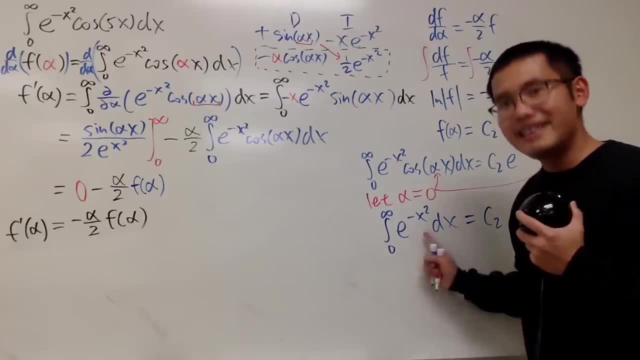 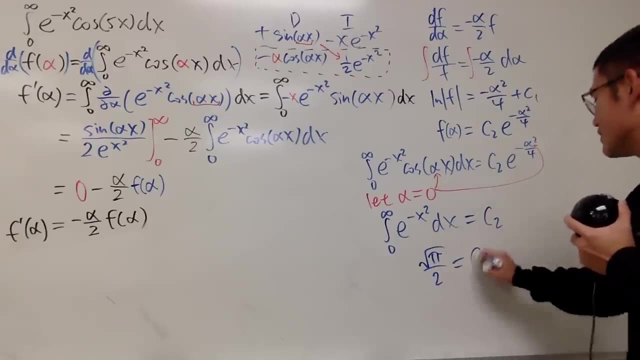 so that's very nice. And now, what's this? The Gaussian integral? This right here is just half of that right. So this right here is famously equal to square root of pi over 2, which is the C2 right there.